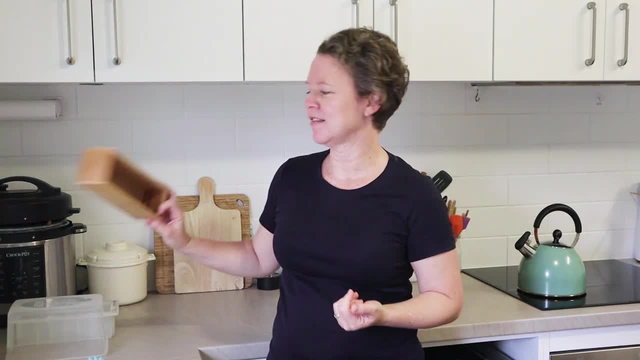 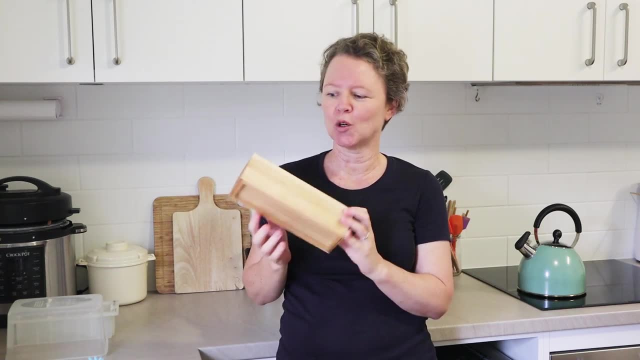 their soap. You know we use all sorts of containers. like you know, this style is one of my favorite, and this is the bamboo drawer liner from Kmart. so it's not designed for soap making at all, but it makes a really good soap mold. So once 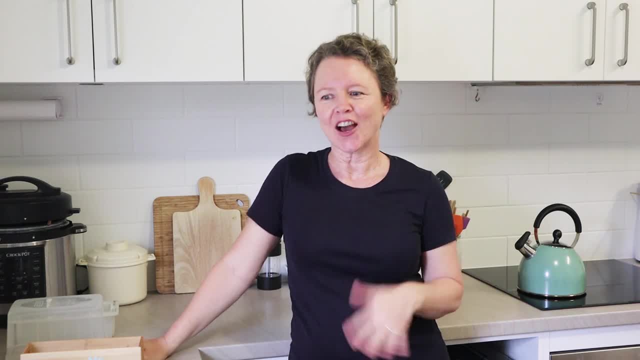 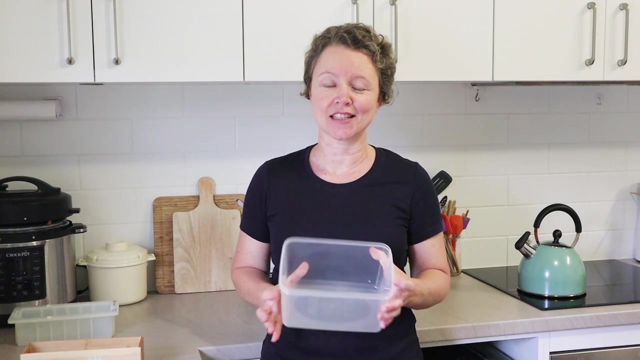 you have learned how to calculate the capacity of your soap molds and work out soap recipes to fit them perfectly. you can make your soap in anything that you like. So, to get started, I just want to start with the most easiest ones to calculate, and these are molds that I use for soap making. 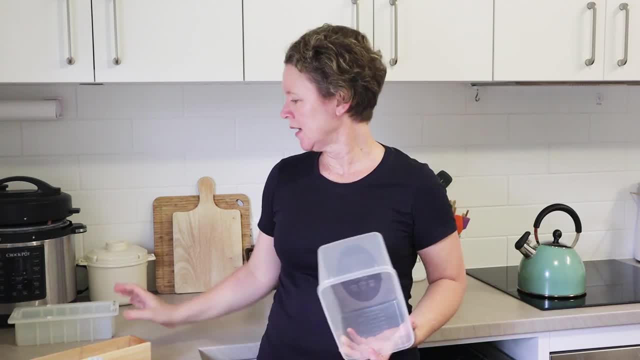 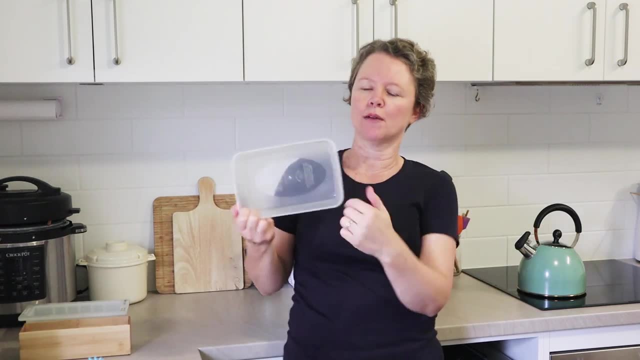 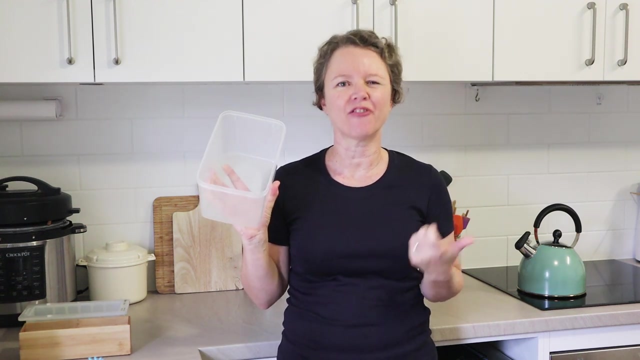 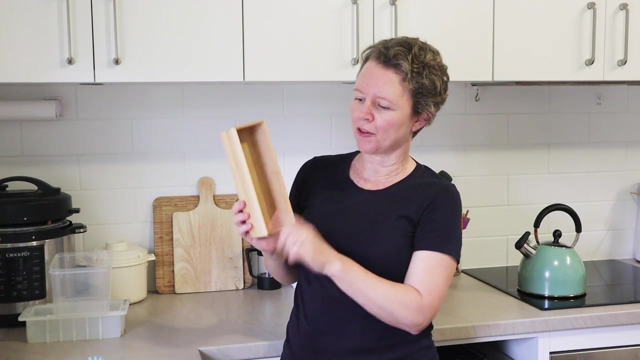 They are basically rectangular in shape or square, something like this, yeah, anything like this. even this one has rounded corners. it still works. You'll be able to take the basic dimensions of this and calculate them fairly accurately. So what we do, I'm going to use this one as an example throughout. 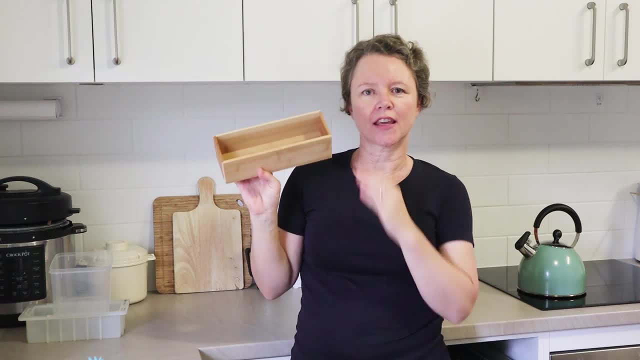 the video What you do to calculate the capacity. so this one is a little bit smaller than the other one. So what I'm going to do is I'm going to use this one as an example throughout the video: what you do to calculate the capacity. so this: 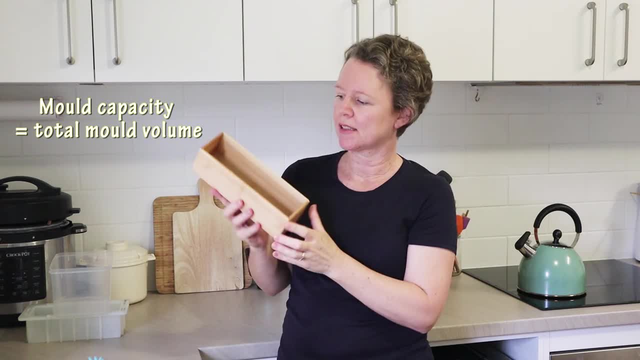 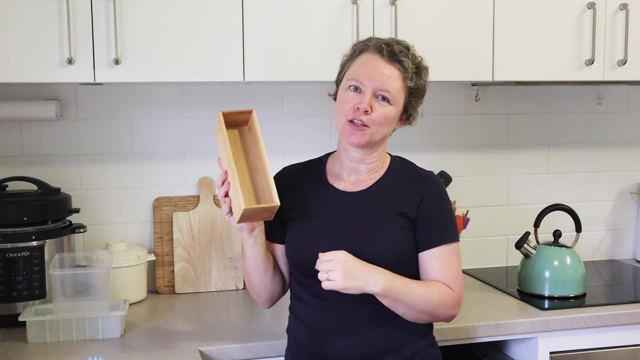 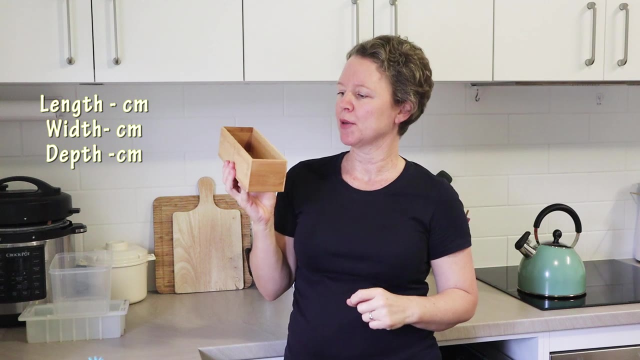 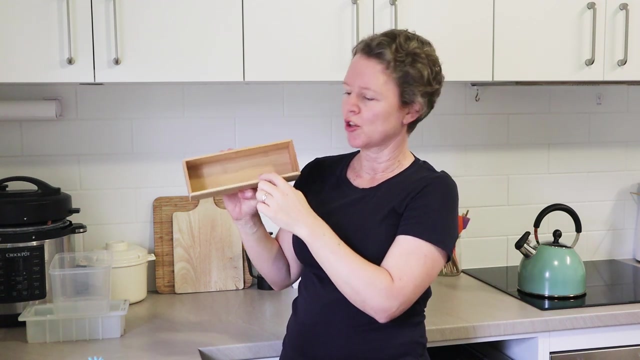 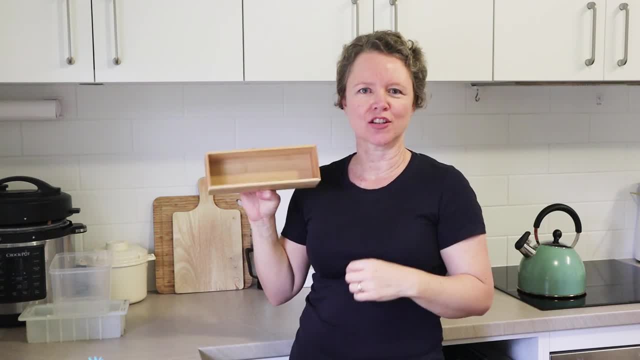 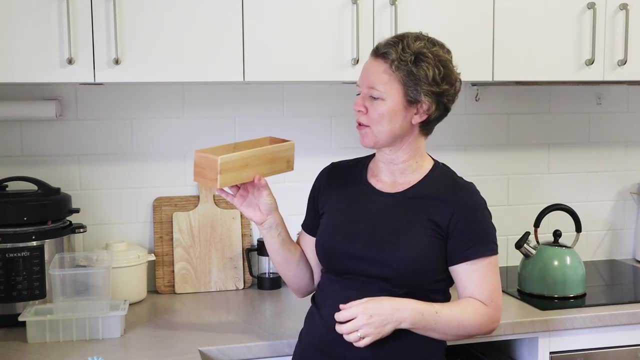 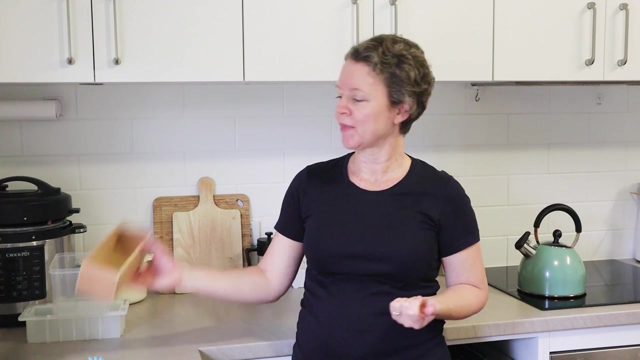 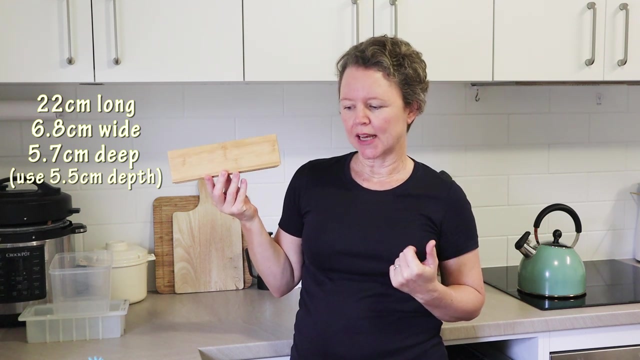 the inside dimension. that's the accurate one, that's going to reflect where your soap is actually sitting. So take the inside measurements of those three- length, width and depth- and then what you do is you basically just multiply those three. So in the case of this mould, this mould is 22cm long, 6.8cm wide and 5.7cm deep. 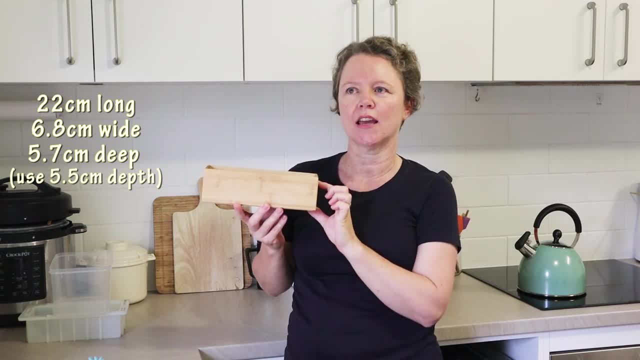 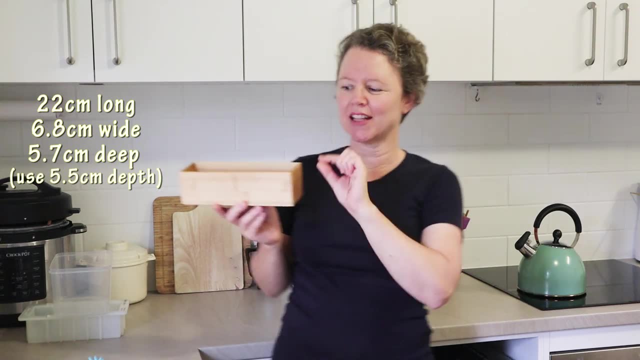 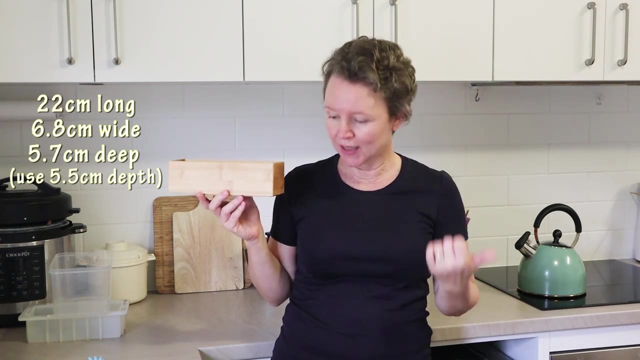 Now for this calculation. I actually say, instead of 5.7cm deep, I would calculate it at 5.5cm deep, and that's because you just want a little bit of a gap at the top. You don't want your soap to be completely overflowing or completely filling the mould. 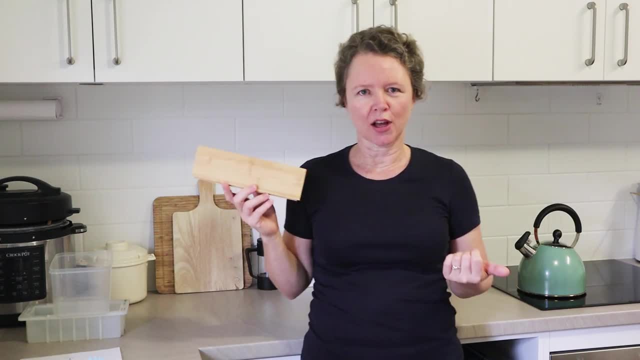 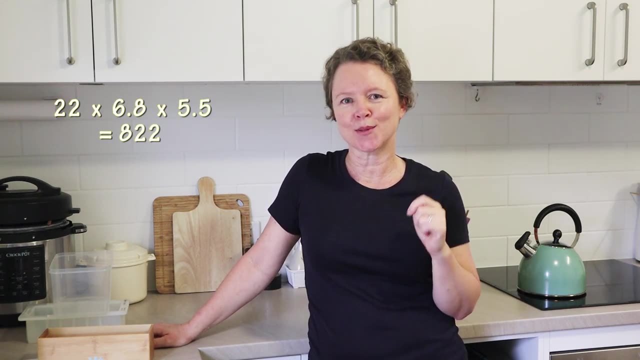 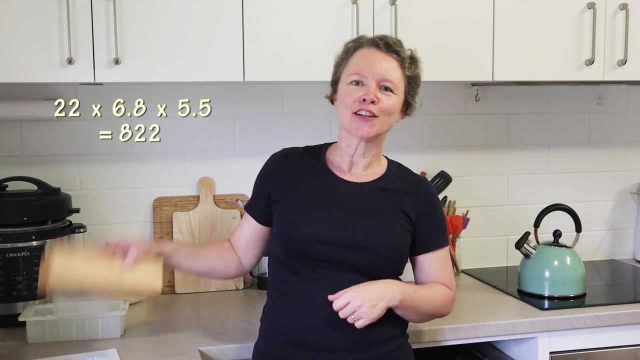 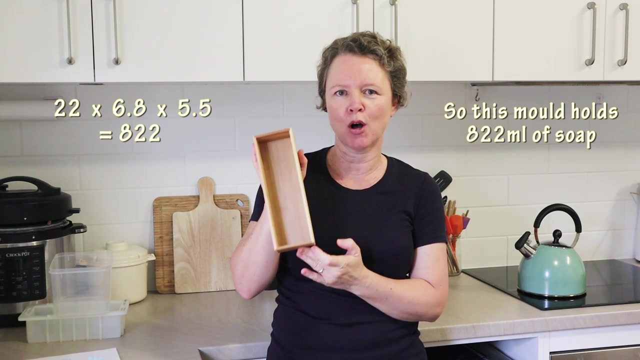 So once you have done that, you just multiply those three values, So you put into your calculator 22 times 6.8 times 5.5, and you come out with the number 822.. Now 822, that is the amount of millilitres of soap that will fit into this mould completely, almost to the top. 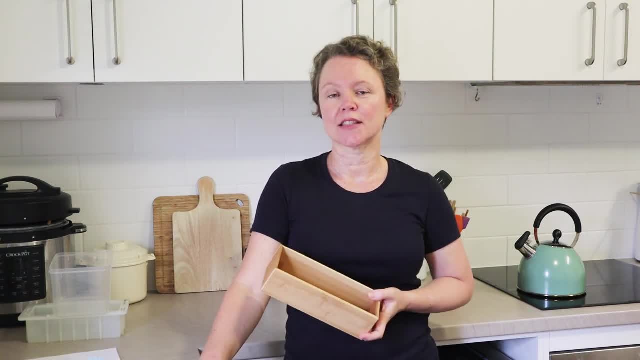 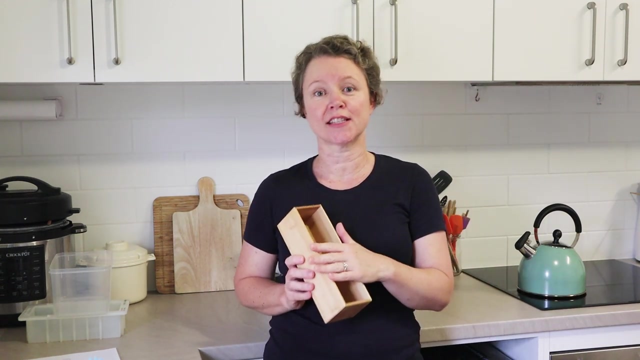 Now I've calculated these using the metric system and you can use the Imperial or the US customary unit measurement system when you're working out your soap recipes. but for calculation- calculating this- the metric system is really handy because in the metric system 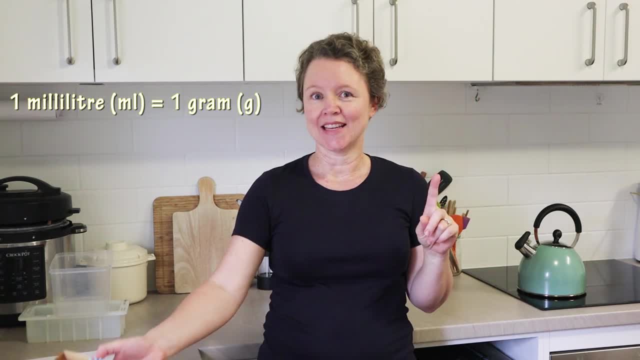 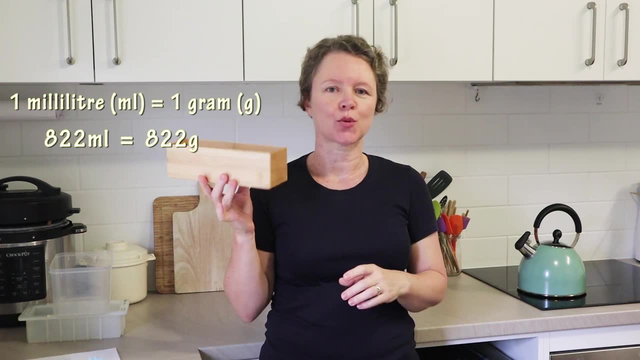 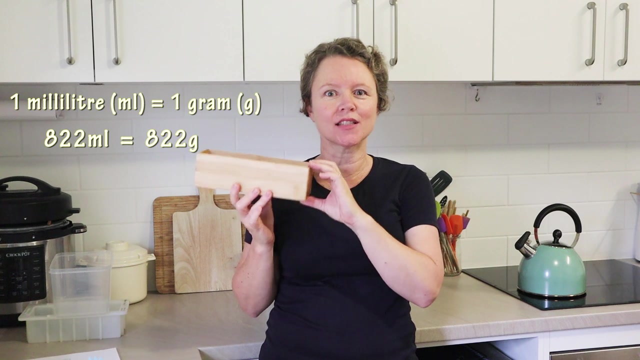 one millilitre of water weighs one gram, So it's really easy. Once you know the volume capacity- so 822mm- I then know that this mould will hold 822g of soap. So once I've got that weight measurement, that I know what this will hold. 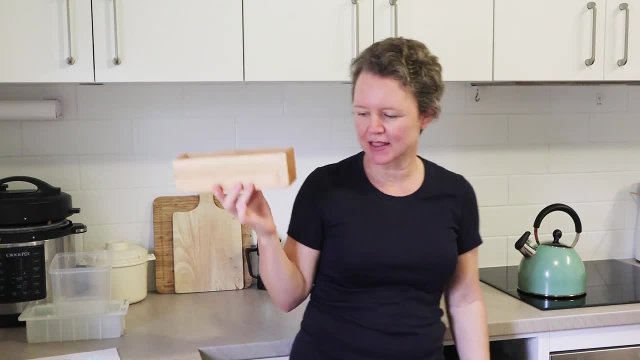 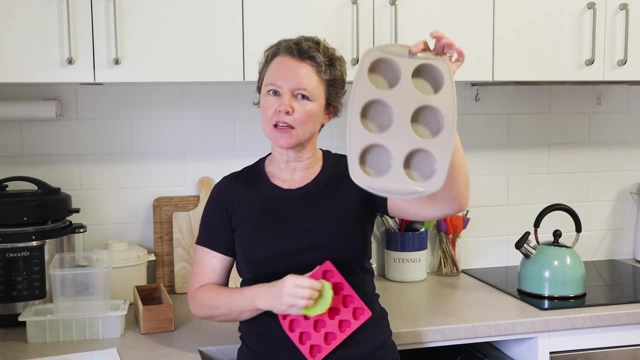 then it's easy to work out the rest. I hope that makes sense. The other thing is: what about irregular shaped moulds? What if you're using silicone moulds like this or even this, or even single little cupcake moulds and things like that? 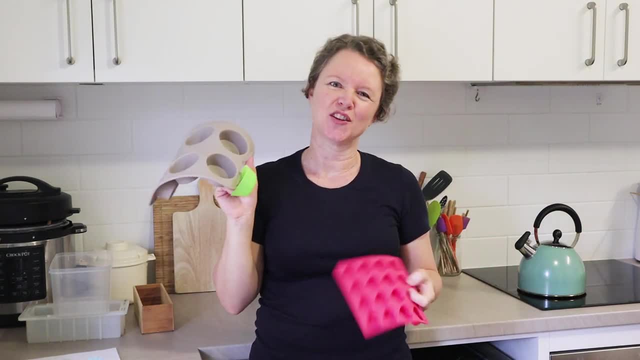 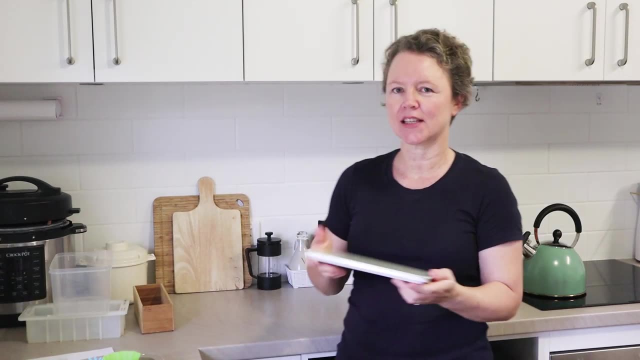 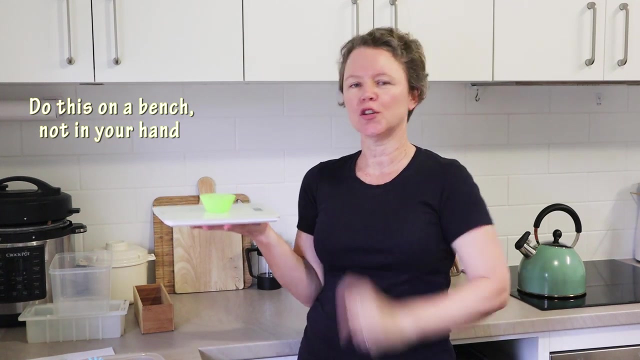 They're easy to work out. so obviously you can't use a ruler and take the dimensions and multiply them. The best way to work out the volume for those moulds is with your scale. So grab your scale, put your mould on your scale. 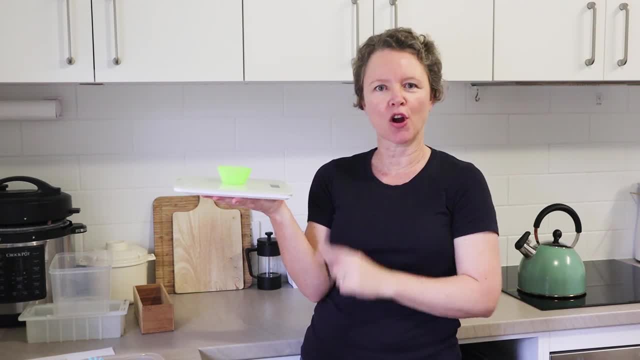 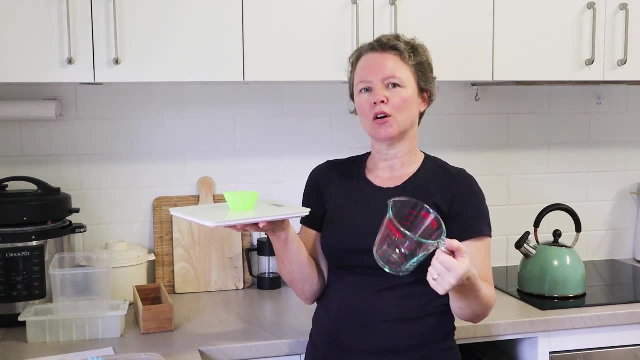 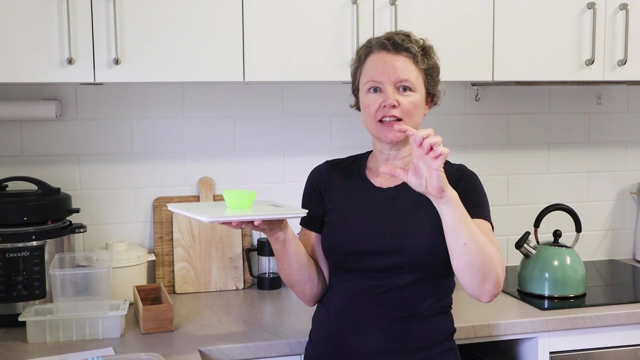 zero it out. so make sure it says zero with the mould on the scale and then just get some water and pour it into the mould until you reach the level that you want your soap to come up to and take what that reading is And that is going to be your soap volume in weight. 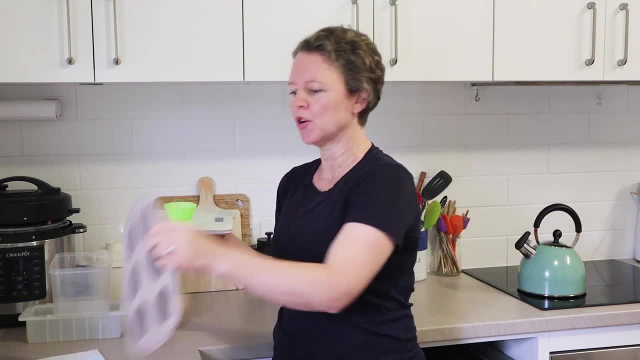 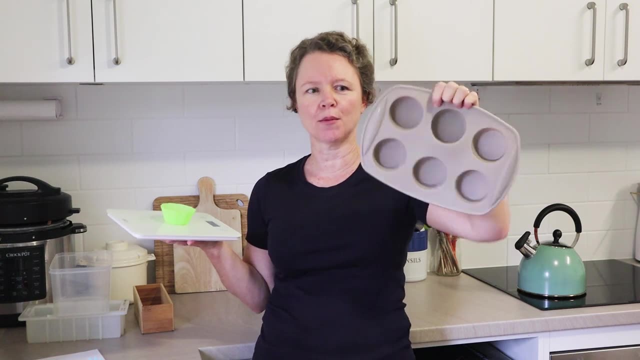 So that's the best way to work that out. If you're using one of these, you can just do one and then multiply it by six to get your total mould capacity if you want to fill up this whole mould, or multiply it by 12 if you're using two. 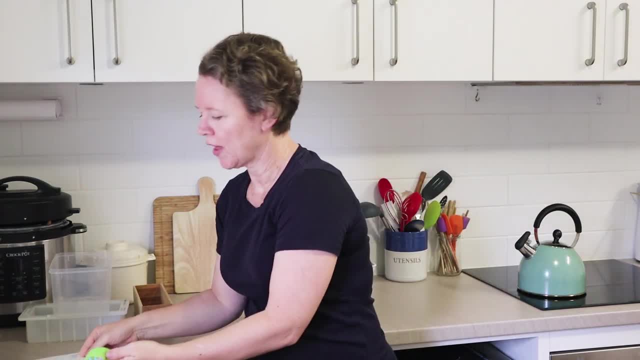 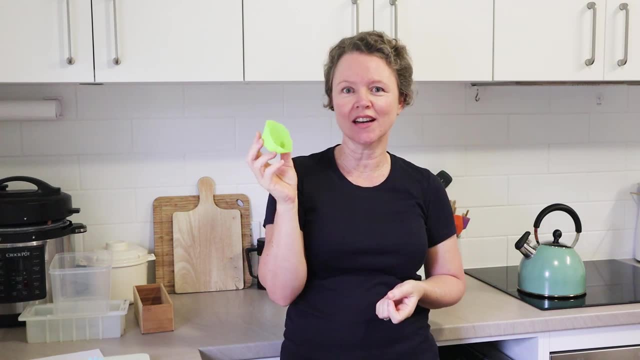 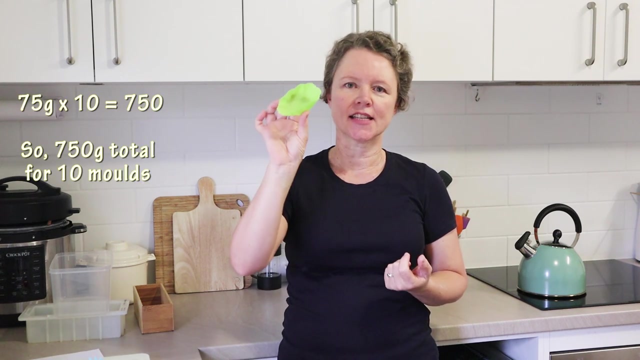 I pre-weighed this one. I know that this mould holds 75 millilitres or 75 grams of water, so I know that that's going to hold pretty close to 75 grams of soap And say if I had 10 of those. I would just multiply that by 10 and get 750 grams. So 750 grams is my total soap batch volume that I would need if I had 10 of these. I hope you're following me here. It is a little bit technical. 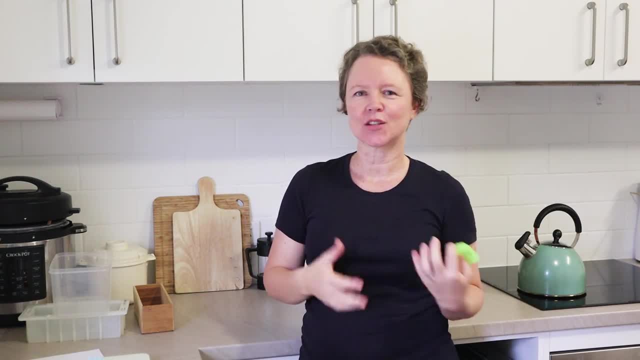 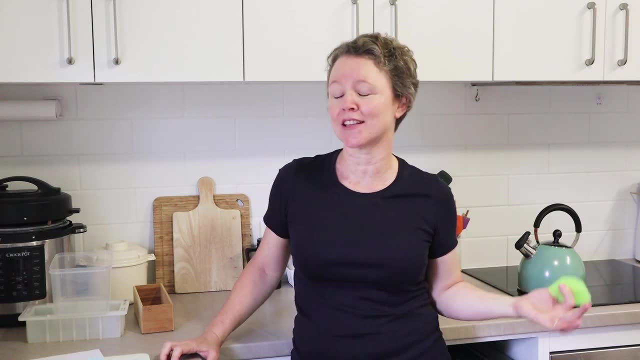 but I find that these sorts of technical subjects, these are the things that people struggle with, and part of what I really want to do with this channel on the soap making side of things, is explain as many of these things as I can, because once you get this stuff, 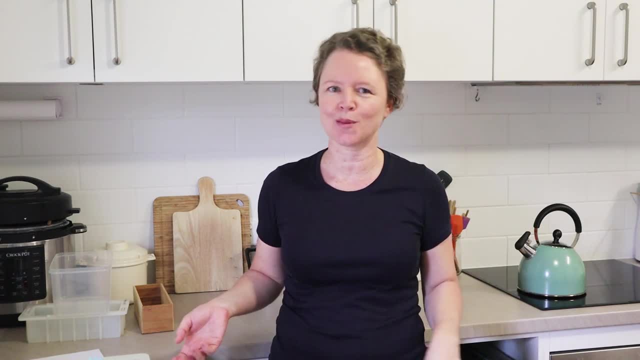 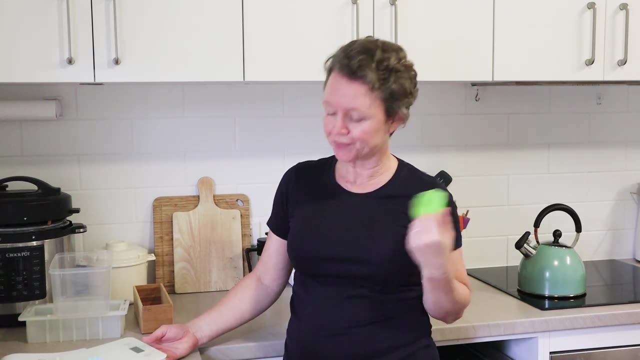 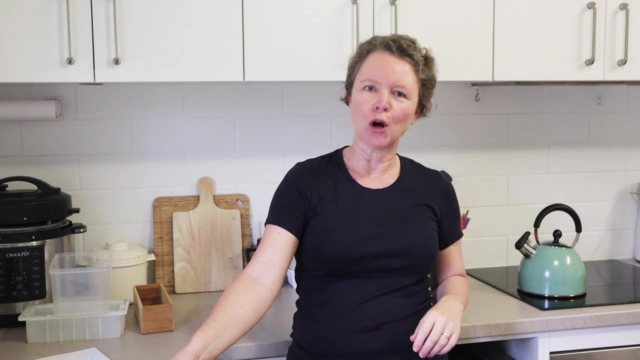 you can do whatever you like and you're not at the whim of other people's recipes and dimensions and measurements and things. You can really customise what you're doing to fit your equipment. So okay, Once you have got the total mould volume, 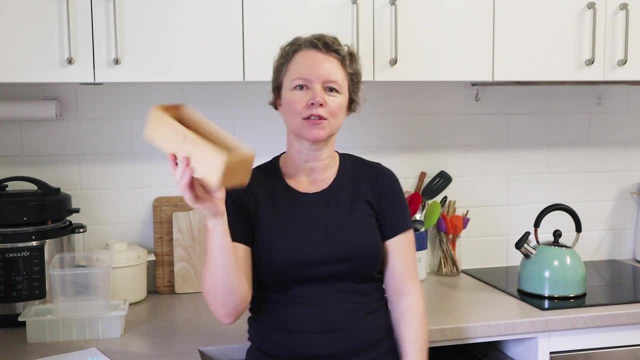 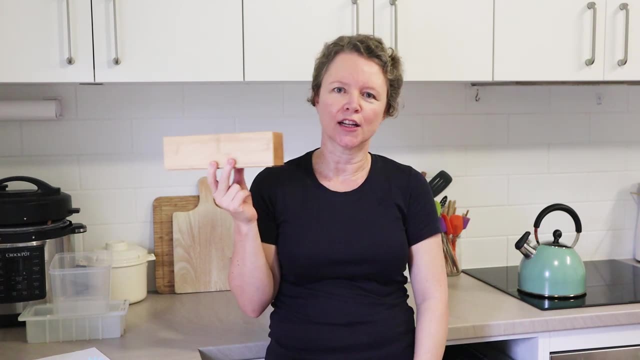 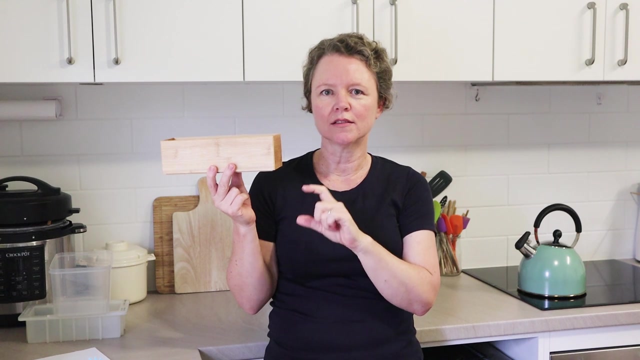 and I'm going to go back to this one, because this one's our example. So this one holds 822 grams. So it's going to hold 822 grams of soap, Just on that water and oil, which is mostly what soap is. 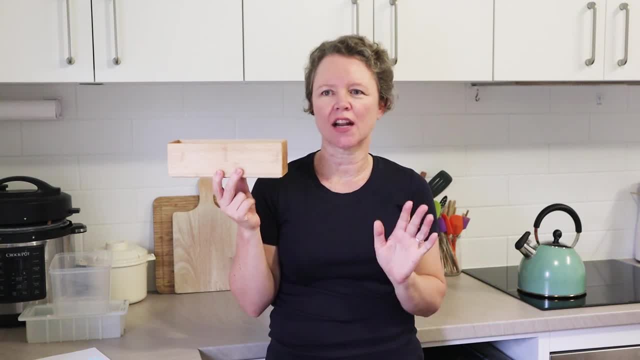 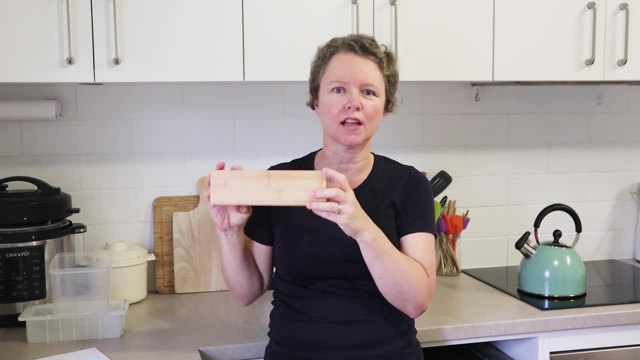 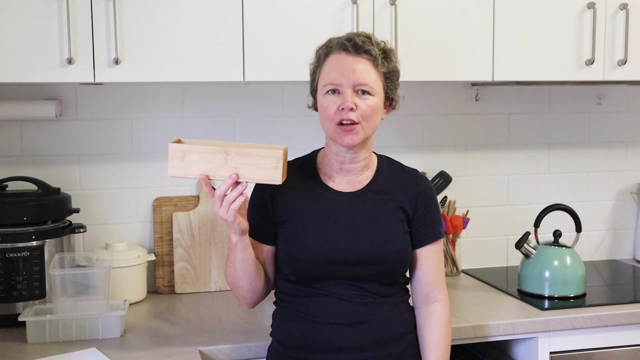 do weigh slightly different amounts, but it's not enough to make it really inaccurate. So, just whatever the capacity is in water, like in millilitres, you can just pretend that it's going to be the same as your soap batter, because it'll be very close. 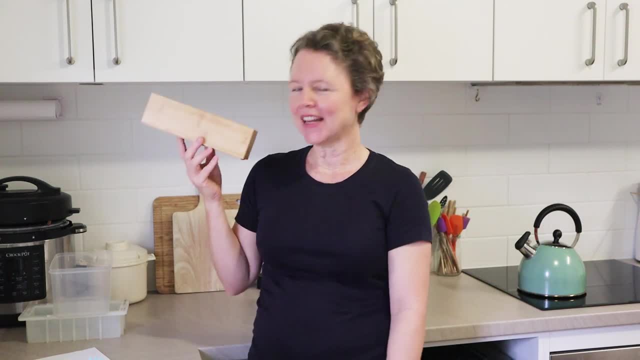 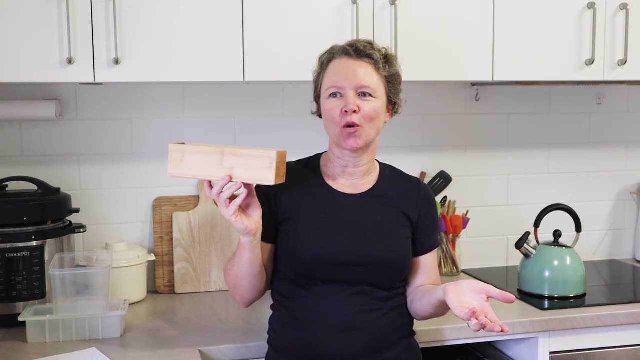 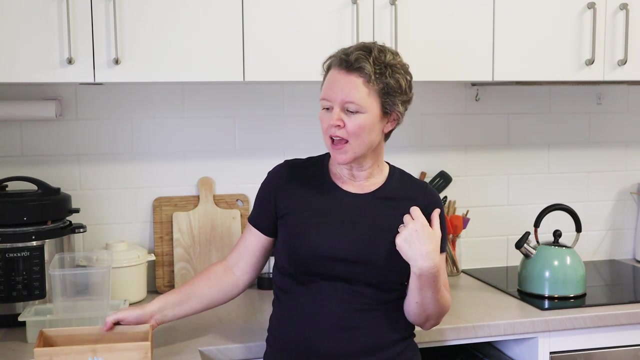 I hope I haven't confused you all. Okay, Now, once you've got the total soap mould volume, the easiest way to work out your soap recipe to fit your mould is to use a little bit of a formula that I've worked out. 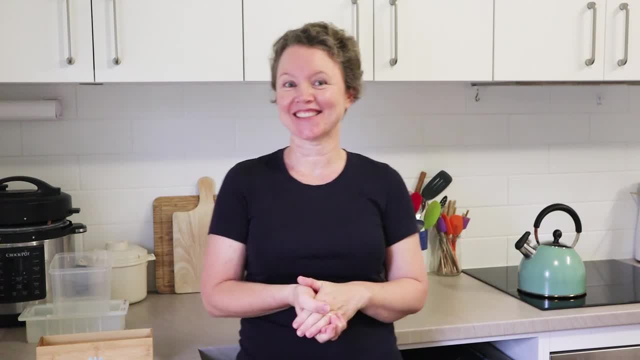 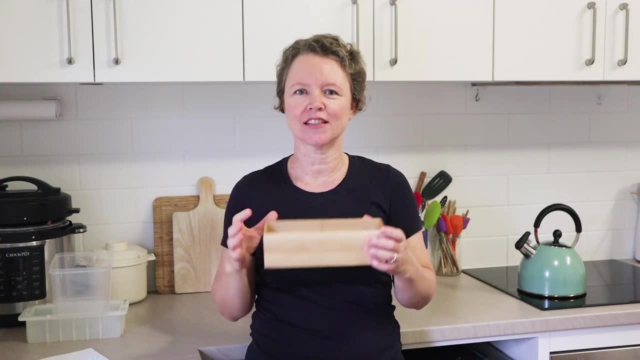 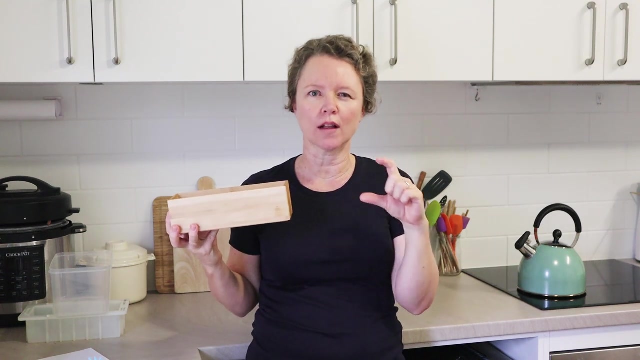 Now my formula is this and it works Here. it is To work out a soap batch size for any given mould. your oil batch size for your recipe, so just the main oil part of your recipe, should be about 70%. 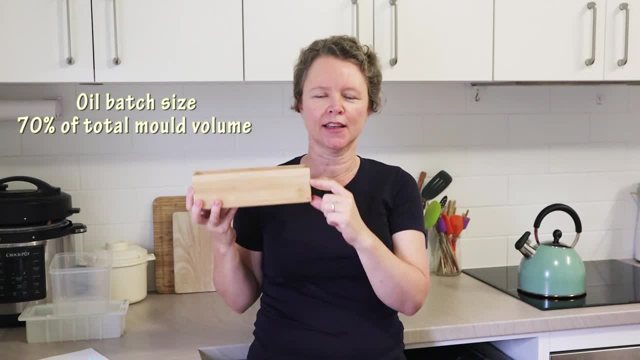 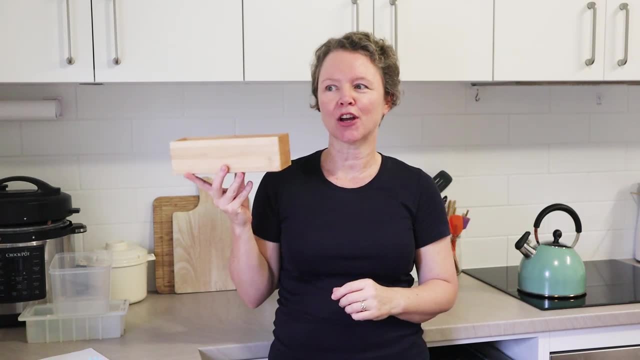 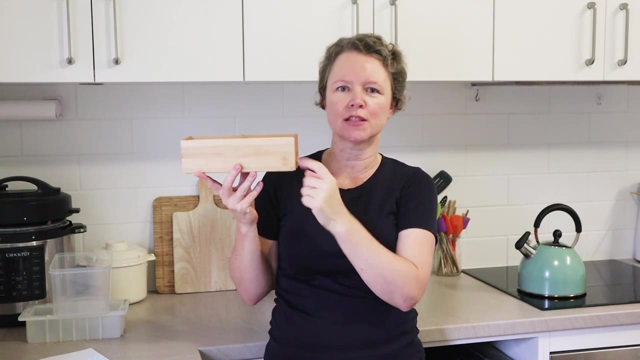 of your total soap mould capacity. I hope that makes sense. So for this mould to work out a soap recipe, I'm going to calculate my recipe based on an oil size for the recipe. that is 70% of this mould capacity. So 70% of this total capacity. 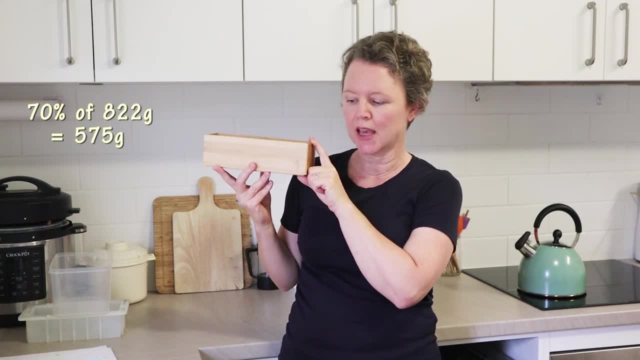 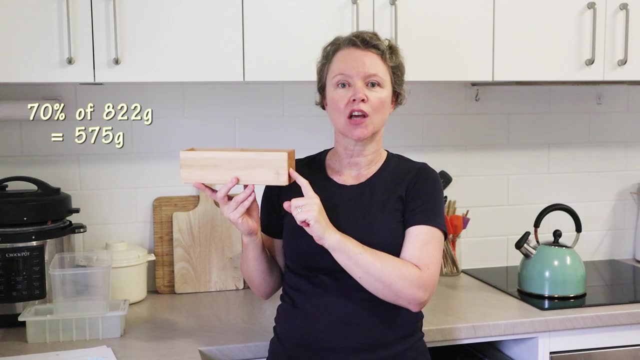 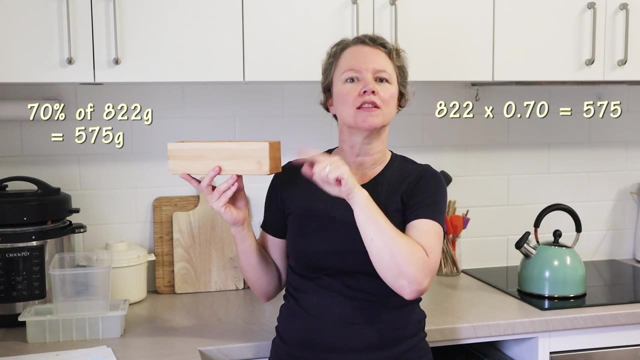 which was 822 grams, is 575 grams of oil. And to work that out it's easy: Just get your calculator type in: 822,, 822 grams, multiplied by 0.70, and that will give you 70%. 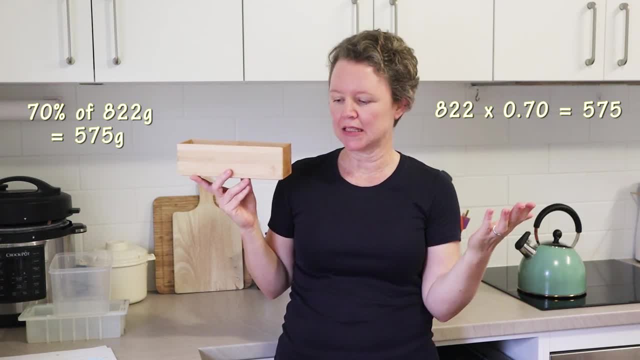 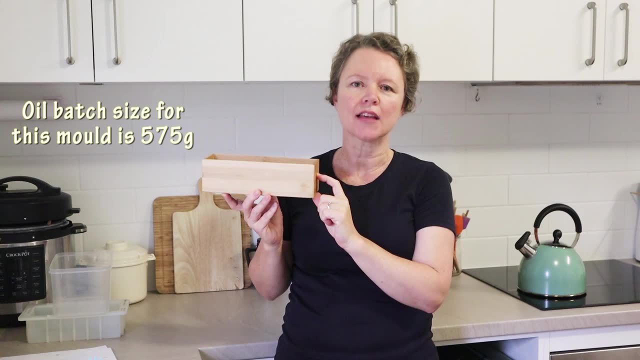 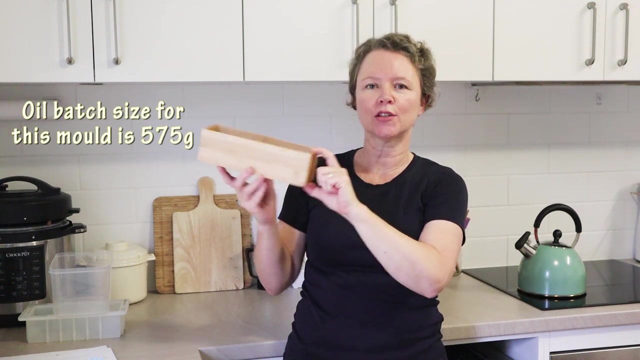 of the 822 grams. It's really easy. So 575 grams is going to be my 70% and I'm going to use that then in my soap calculator as my oil batch size and that will give me a recipe that fills this mould wonderfully. 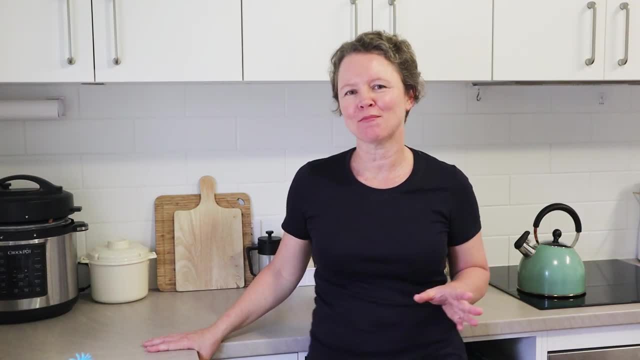 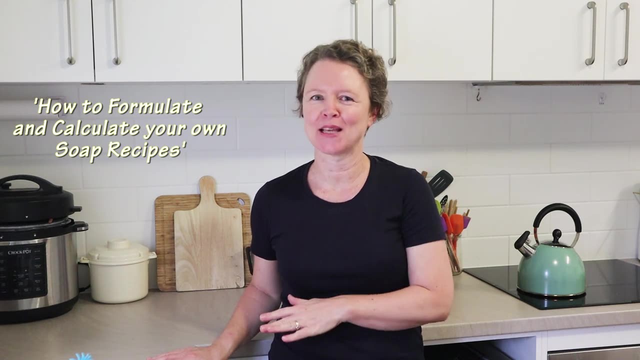 If none of this is making sense to you, please check out my video called How to Formulate and Calculate Your Own Soap Recipes. Some of the concepts that I'm talking about in this video won't make sense to you if you aren't familiar with calculating. 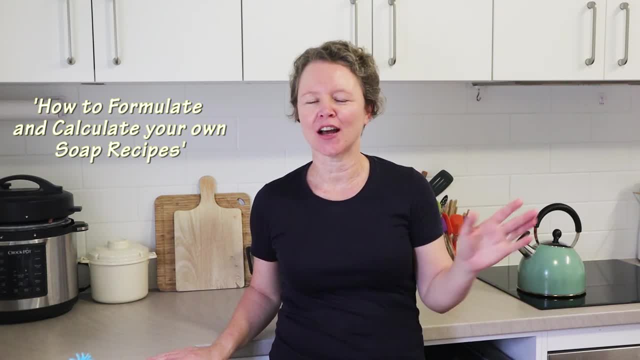 your own soap recipes. Check that video out. I'll put a link to it in the description box. Once you've seen that one and are familiar with the concepts, it'll become a lot easier. Now there are some other variables to consider. 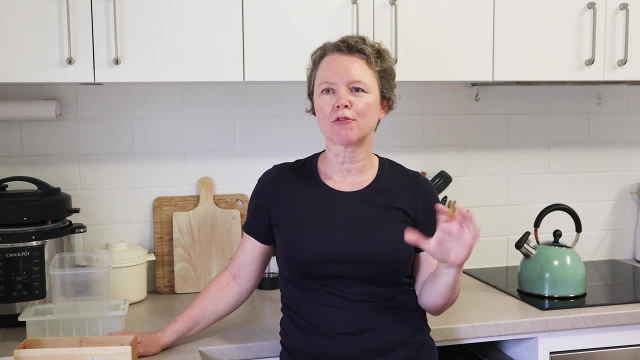 I make my soaps with a reasonably low water amount in my recipes. The 70% formula that I've just talked about works really well with medium to low water soaps. If you're using a lot of water in your soap like a high amount of water. SoapCalc and a lot of soap calculators default at 38% water of the total oil amount in your recipe, which equates to about a 25% lye concentration solution. I don't make soaps with that much water in them most of the time. 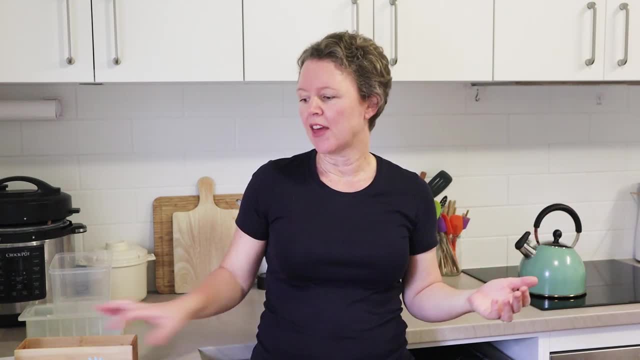 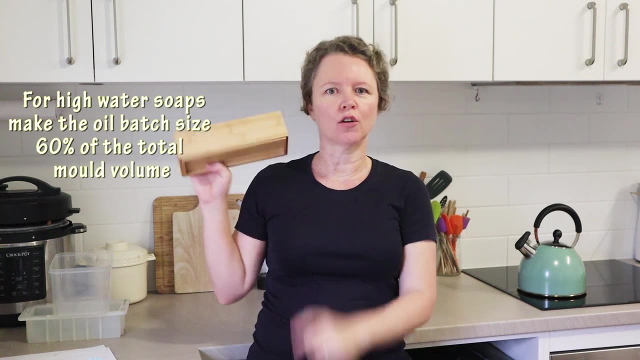 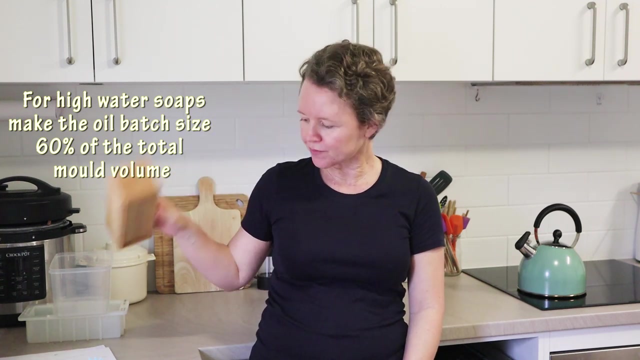 If you're going to use a high water soap like that, then you would probably want to try 60%. Make your oil batch size 60% of your total soap mold volume. That will account for the extra water in your recipe. I hope that all makes sense. 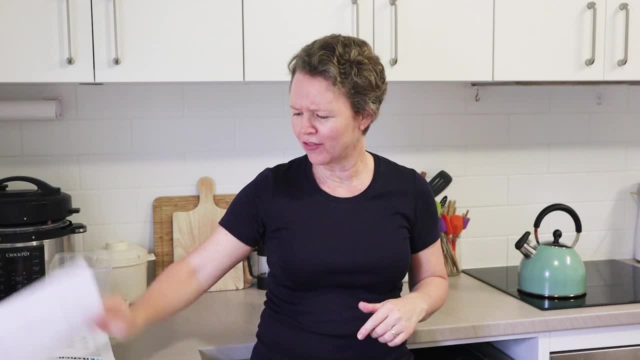 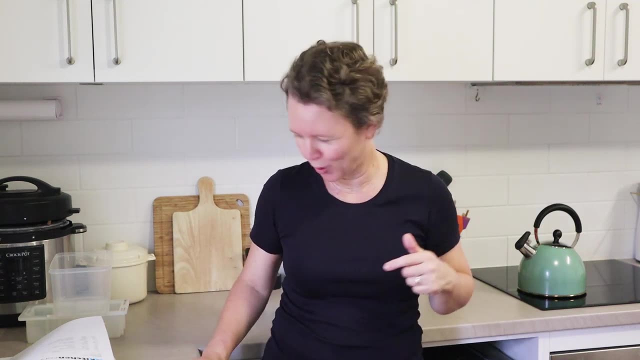 Let me just see if I've forgotten anything. I don't think I have. Yeah, that's it. There's nothing else to it. So just a bit of a recap. So what you do first is decide on your mold, Work out the total volume of your mold. 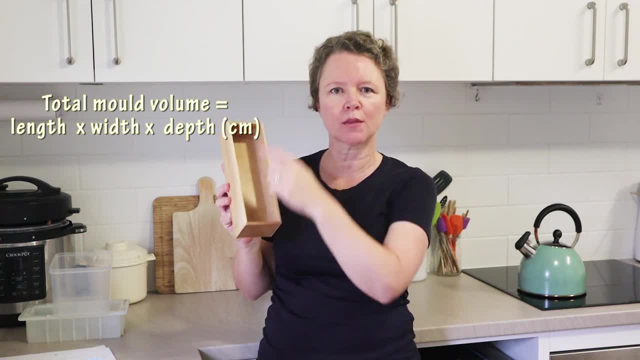 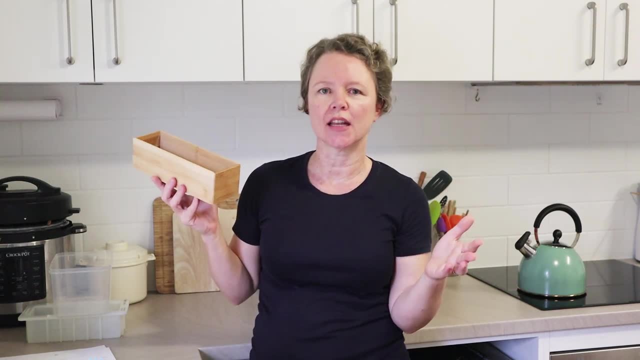 If it's square or rectangular, multiply the width by the length, by the depth, to give you the total milliliter capacity. And if you're doing that in grams, then that will. if you're doing that in milliliters, that will equate to the number of grams. 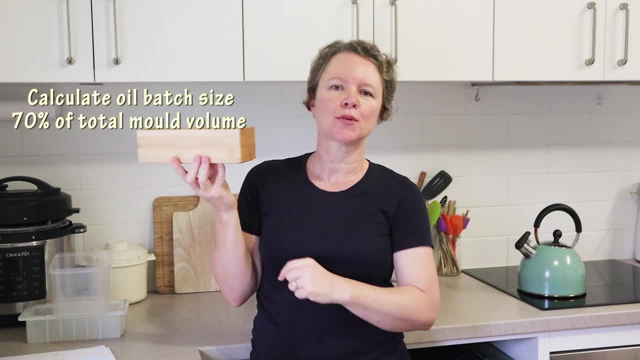 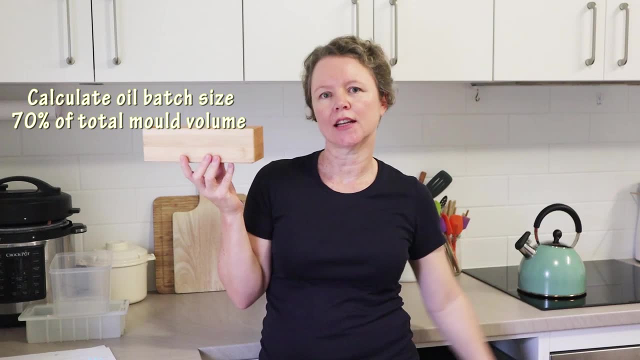 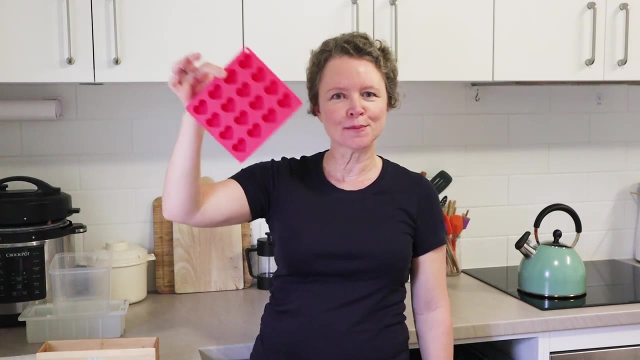 that it will hold And then calculate 70% of that and that is your oil batch size for your soap recipe that you're going to calculate in SoapCalc or whatever soap calculator that you're using. If you are using random shaped or sized molds, 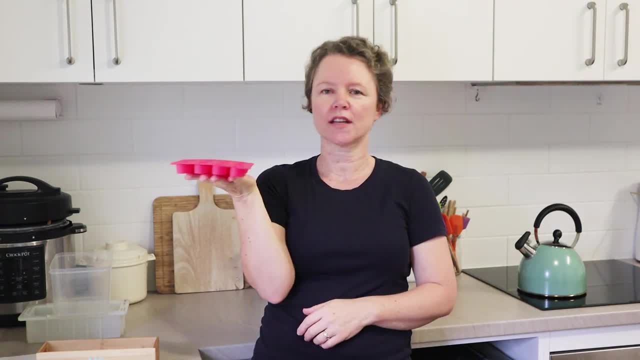 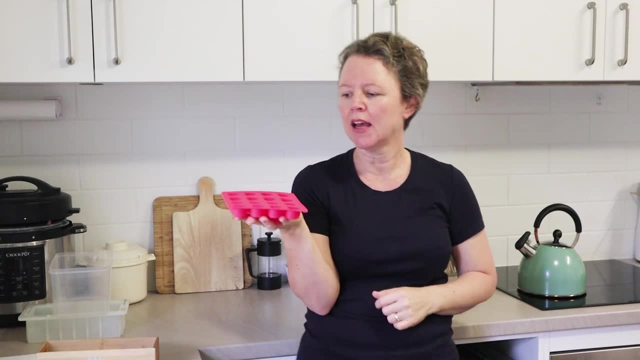 then it's the same. Just use the water and the scale method to work out the total volume. You can just do one and multiply it by however many you need And then, once you've got that total volume amount, multiply it by 70% or 60,. 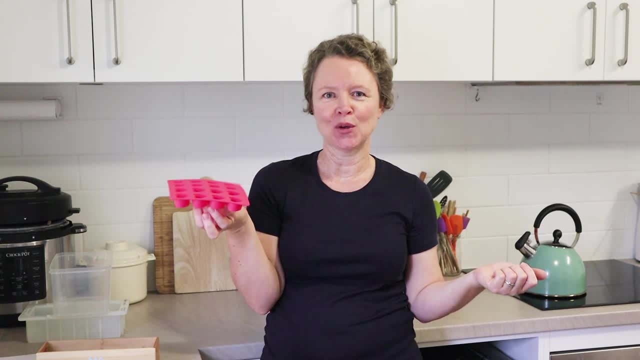 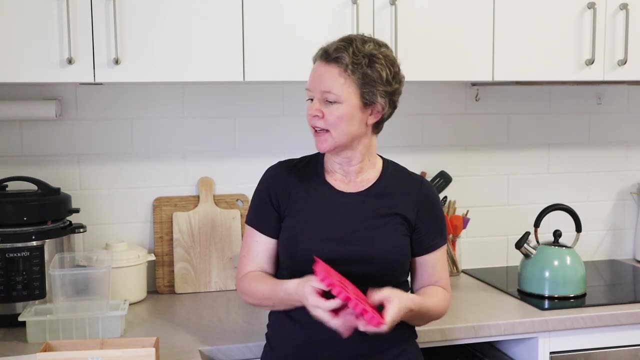 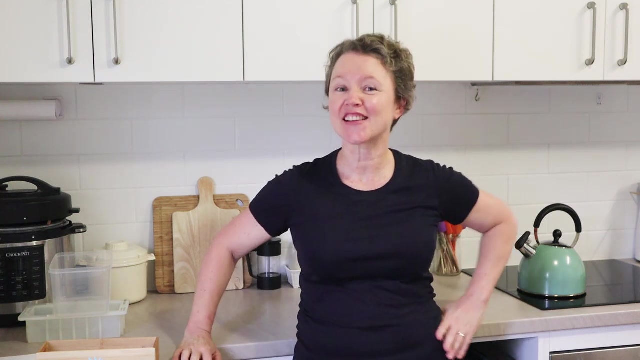 you know, just get 70% or 60% volume amount to put into your calculator as your oil batch amount. So I hope that makes sense to you all. I think I've explained it as best as I possibly can. I've actually filmed this video three times. 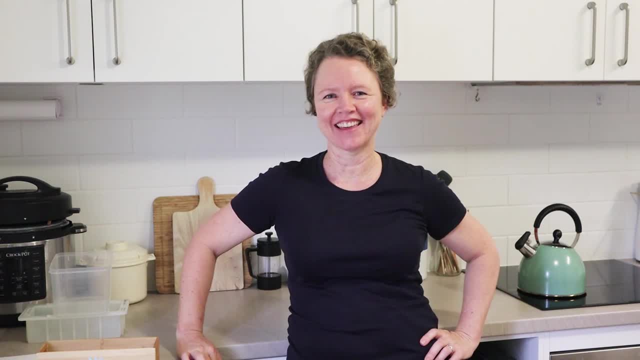 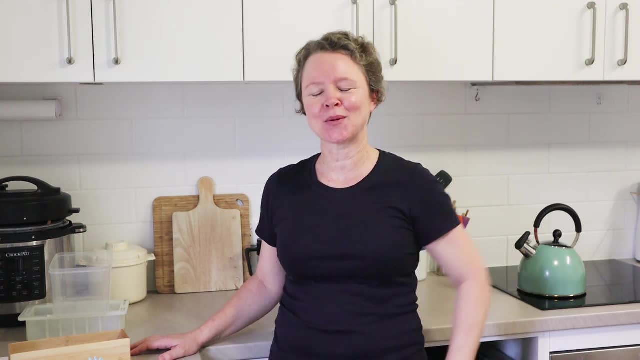 So you know it took me a while to get there. I'm sorry about the sweating. It is boiling hot here. It is summer, It is March in 2020.. And yeah, it's quite warm, so I'm a bit sweaty. 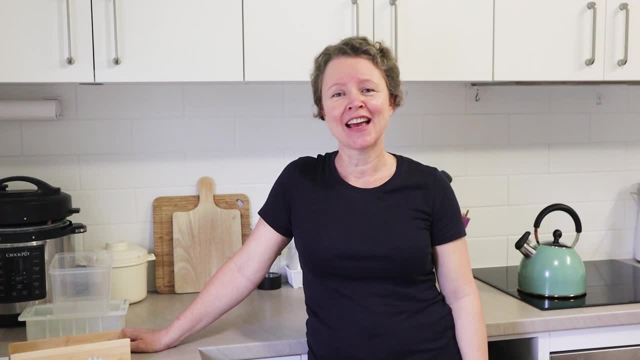 Anyway, I hope you enjoyed the video. everyone, Enjoy your soap making. I will be back for more videos soon, as soon as I can Bye.